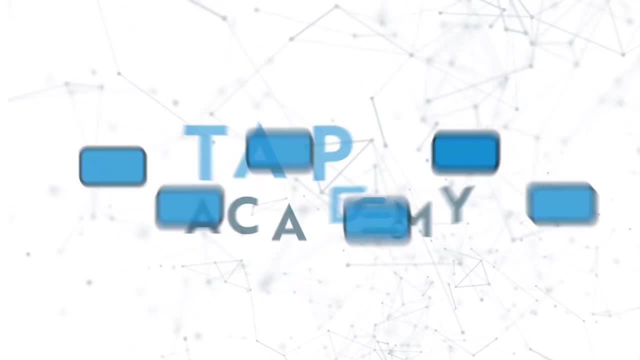 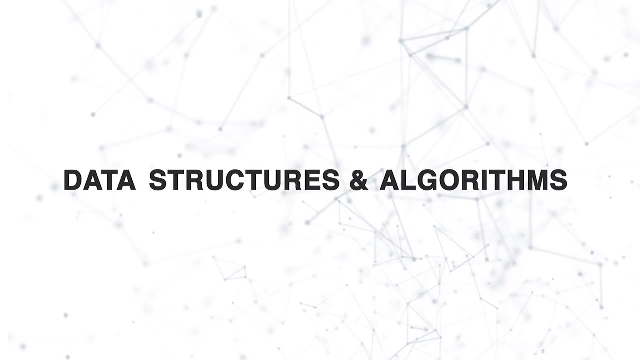 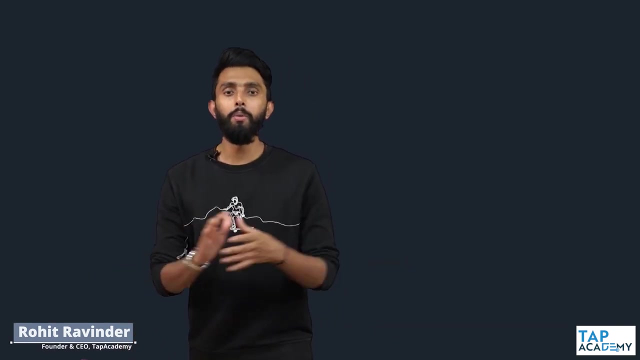 Namaste and welcome back to the DSA classes. Today, my dear friends, we are going to explore a brand new data structure. Of course it is not new, because you have certainly been using it in different ways when you learned either Java or Python, And I am a friend- 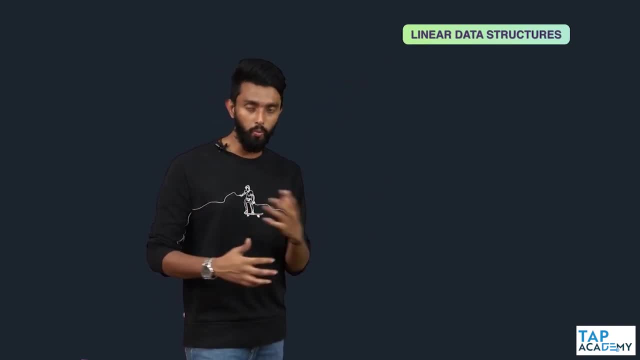 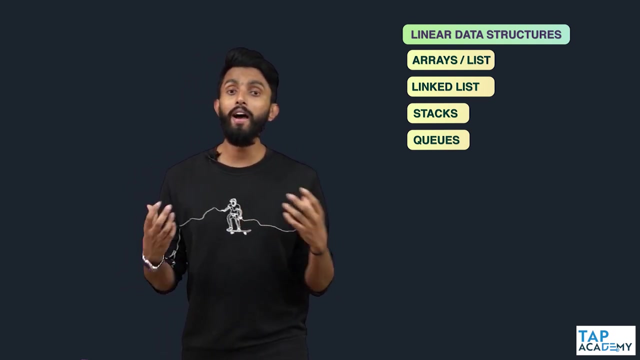 I am talking about the linear data structures. Now, what are the linear data structures? If you ask me, there are four linear data structures: Arrays, or what you call in Python as lists, linked lists, stacks and queues. These are the four data structures. Now why? 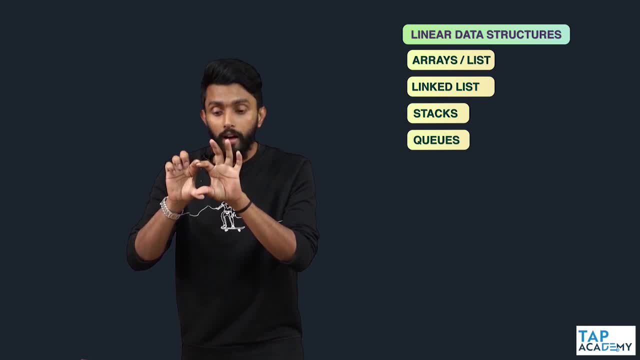 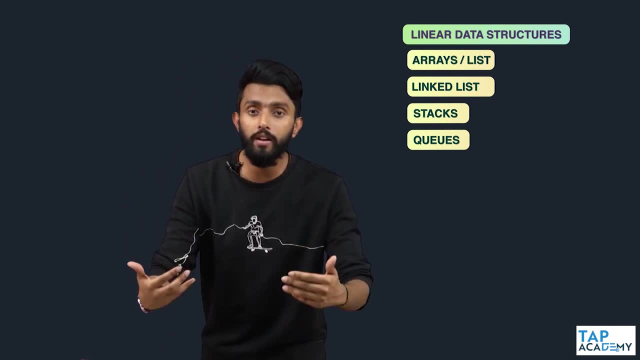 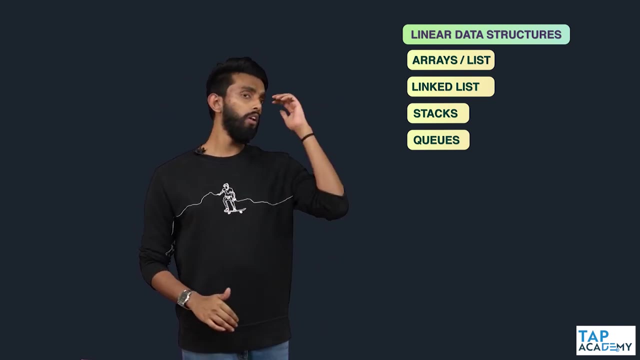 are they called as linear data structures? Because they store data in a contiguous manner: One next to the other. they store the data. That is why they are called as linear data structures. right, More about their properties we will explore in depth, But in order to 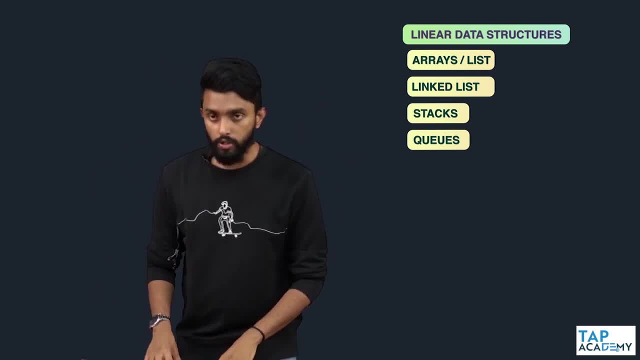 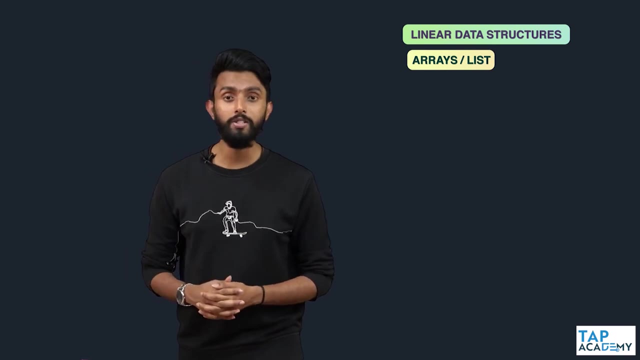 progress to linked lists, and then stacks, then queues. first, the most fundamental data structure which you, as a programmer, are going to be using repeatedly in your life is nothing but your arrays or lists. I hope you are able to think So. let us start arrays and lists. 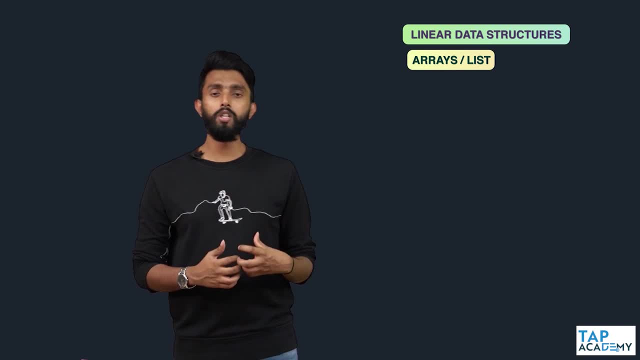 In depth. we shall look at it. okay, So to warm ourselves up, initially I want to be solving some basic programs to get an idea right, Just to warm ourselves up. Then we will tackle all your Google, Microsoft, Amazon problems that can be asked on arrays, right. 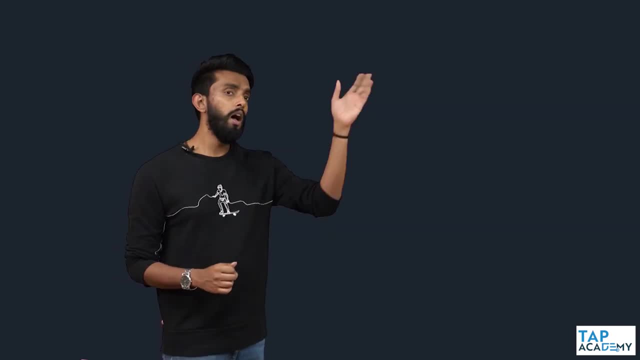 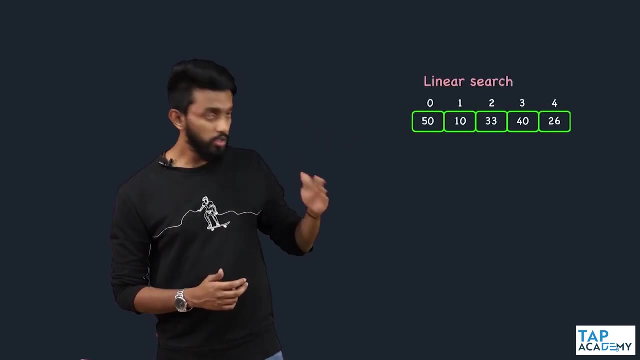 Anyways, first and foremost, what I would like to do is I would like to now write a program to perform linear search. Now, what does linear search mean? Assume this is an array, I want to search for 40, if 40 is there or not, or any element I want to search for. 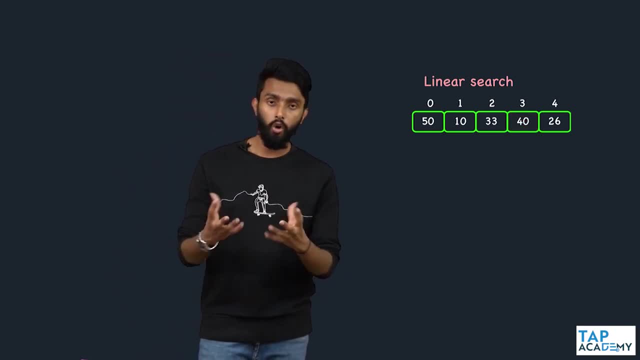 10 for that number. How do you perform search? This is only your concept of linear search. Now, searching is a very important operation. We will be looking at different searching algorithms which are more and more efficient. but let us begin with linear search Now. 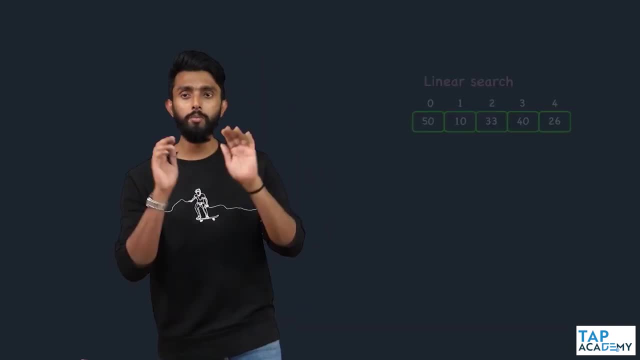 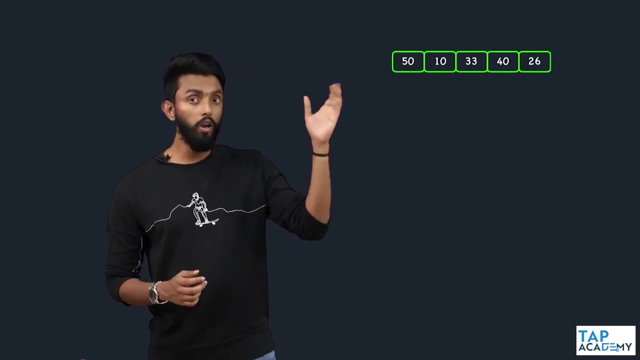 what is the principle or idea behind linear search? It is quite simple, okay. So, basically, what happens in linear search is assume this is the array or list given to me. Now, all of you know, arrays or lists are index-based data structures, right? So if you want to, 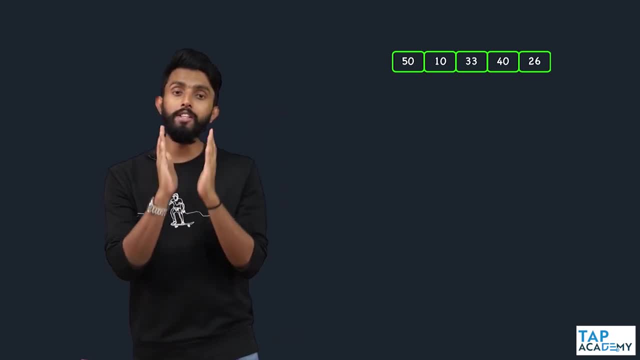 do linear search, you need to have a list of index-based data structures, which means every element or every cell has a position attached with it, has an index attached with it, And you know the indexing that we follow in programming is zero-based indexing, which. 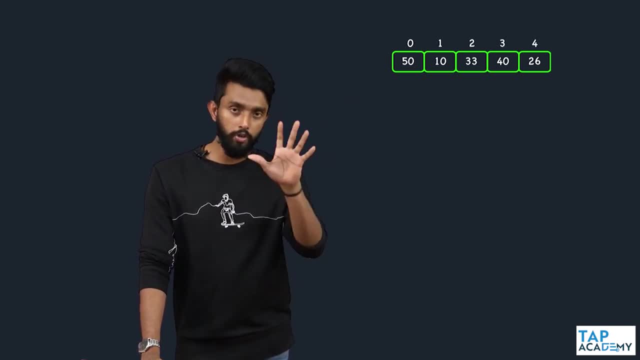 means from zero the index begins and it goes to four, which means I have five elements. Any confusion? Now I will call this as a. Now let us assume I have a variable called as key, inside which I have 40. Now, key is usually the name that we call for linear search. 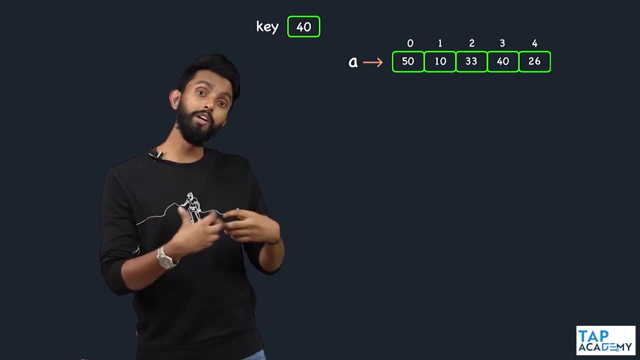 So I will call it for a variable inside which we have that value which we are searching for. That is what is called as key. Any confusion? So I want to search for a key called as 40. Now, how will you do that? Very simple, I will run a loop which begins from the first. 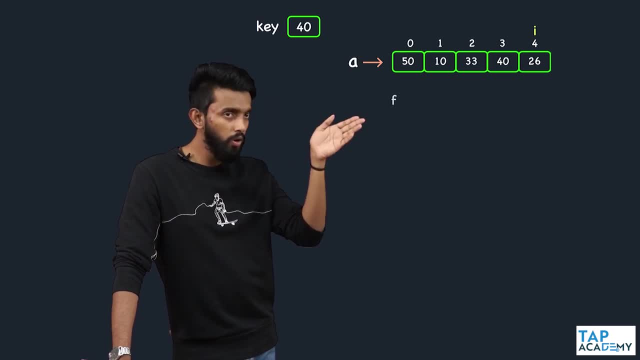 index goes all the way to the last index. How can I write that as code? For i, starting from zero to the length of the array. Length of the array means I am going till the end. Any confusion Now inside that? what will I do? What I will do is I will check if in 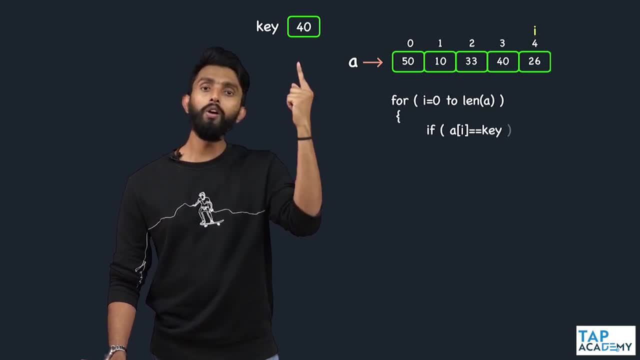 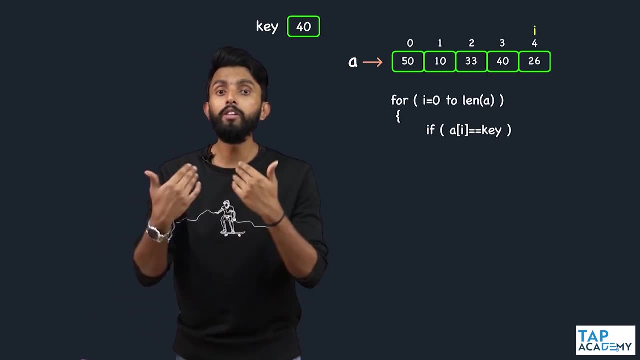 the present at the ith index. So a of i. is that equal to key? I am just checking If it is equal to key. I have found my element and obviously I have to return the position at which the element is present or the index. So the index is in i. So this return i. 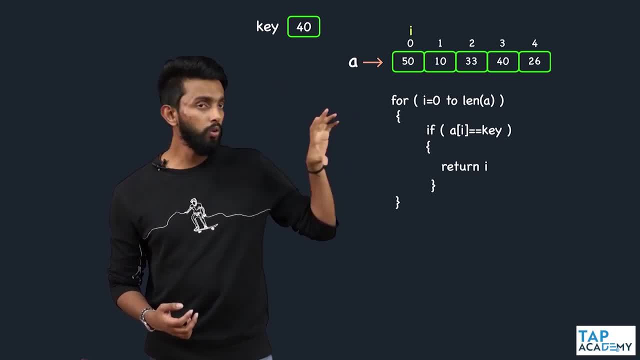 right. So this is the code of what we are trying to do. Now let us assume I run the loop, So i starts from zero. Obviously, if a of i is equal to key, no condition is false. i moves forward. 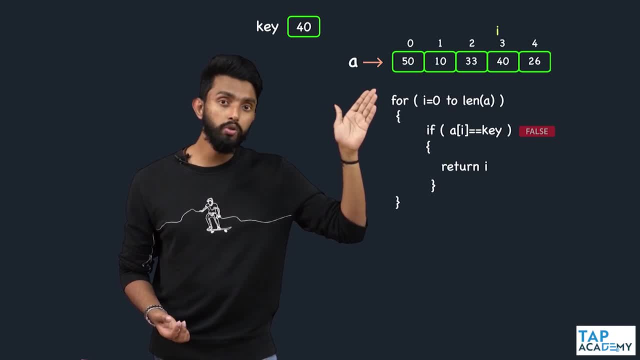 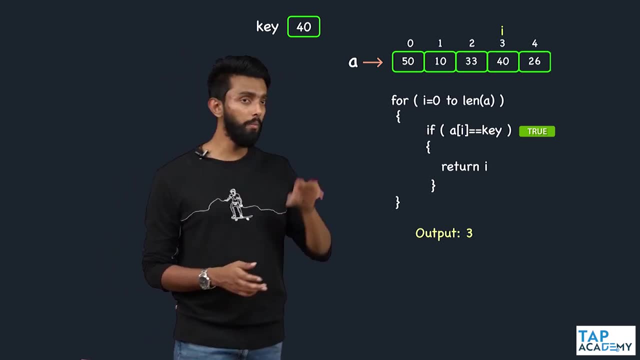 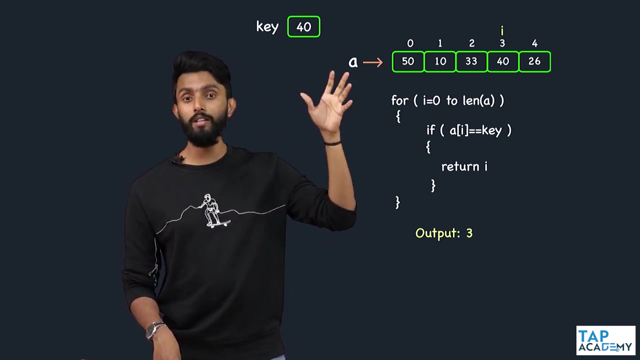 Condition is false. i moves forward. Condition is true, So I will return 3.. It is at the third index. Any confusion till this point in time? Beautiful. Now, this was a case where the particular element is present. But what if it was not present? Well, let us change. 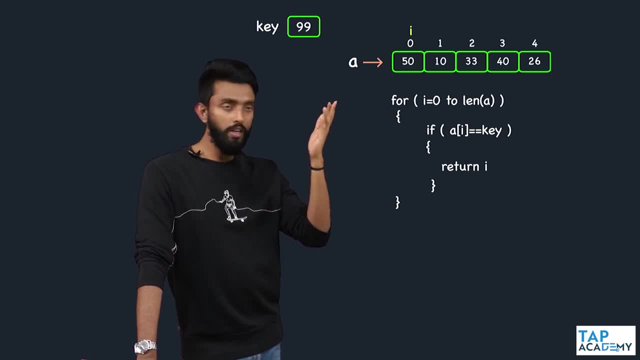 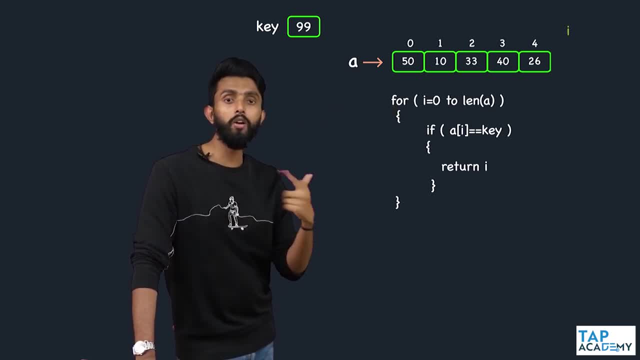 False Again, i will go outside the boundary, So obviously your iteration will stop. So you went the entire length of the array but you did not find 99.. So if the control comes outside the loop and this condition never satisfies, it clearly means that you have. 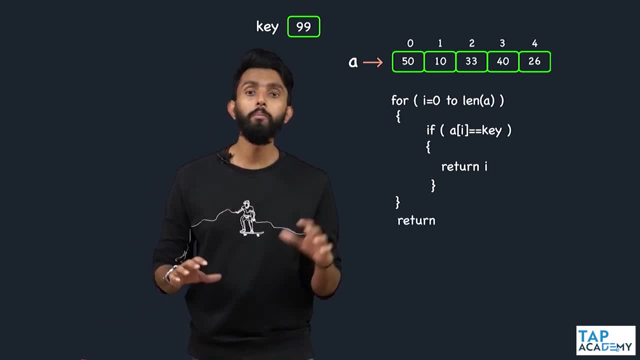 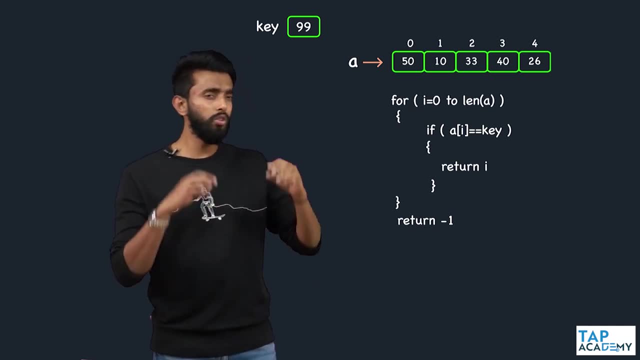 not found the element. Since you have not found the element, I will return minus 1. one. if I return, it means that I have not found the element. So this is the most basic search that you can perform. One thing that you can clearly notice through this example is if 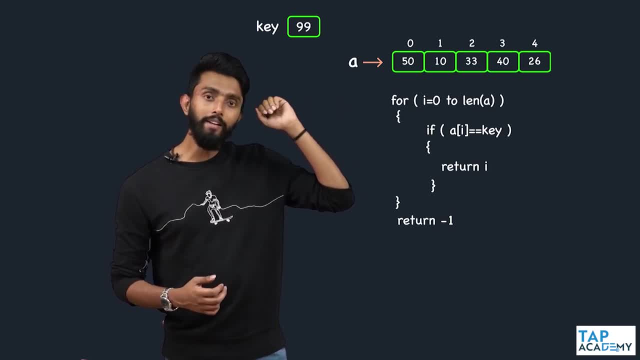 the element you are searching for is not present. you will be iterating through the entire length of the array and keep checking which means this operation you are performing n times. If n is the length of the array, n times you are performing it. How are you able to think? 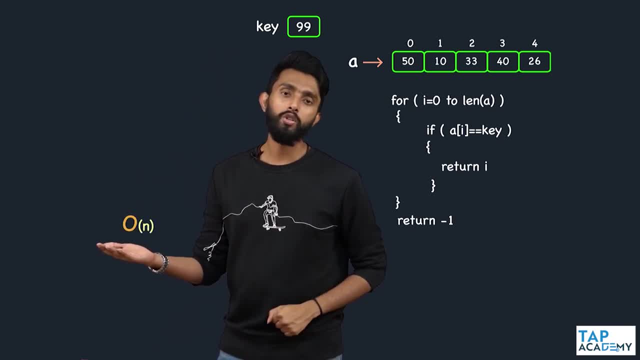 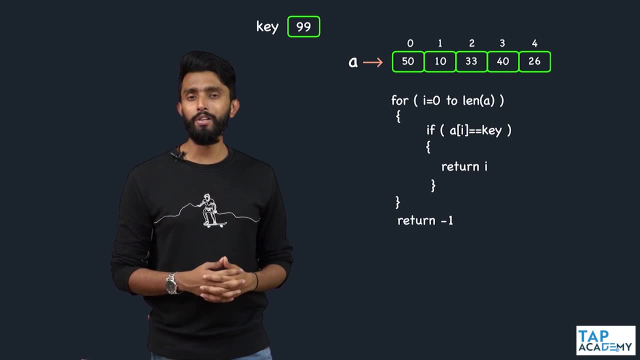 Which means the time complexity is O. Clearly this is not efficient. Are there more efficient searching algorithms? Definitely That. we will look at it later, But this is the time complexity of linear search. Now let's just quickly go write the code, As you can see, 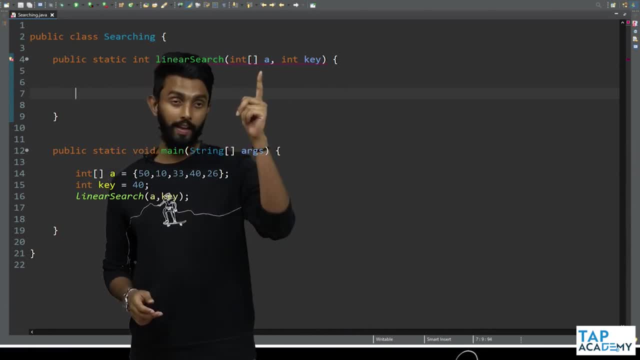 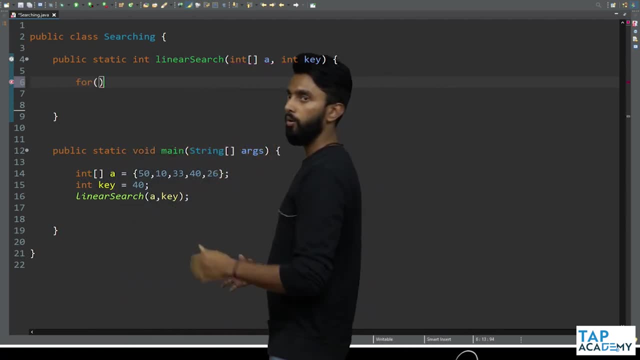 I have a linear search function written which accepts an array A and a key which is again an integer. So inside that I will just run a for loop which is going to iterate over the same time. So I will just run a for loop which is going to iterate over the same time. 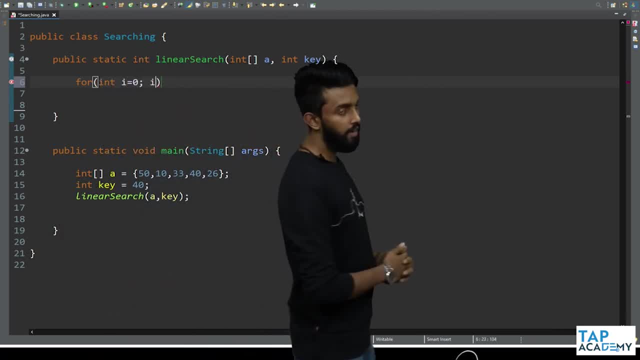 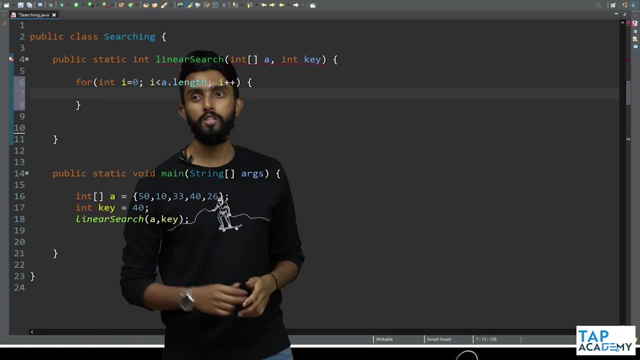 This array: A, So int i equal to 0.. i less than a dot length, i plus plus, And in a set that I'm going to come and I will just now check if in case a of i is equal to the key. If a of i is equal to the key, then clearly you can notice inside of that. I will just 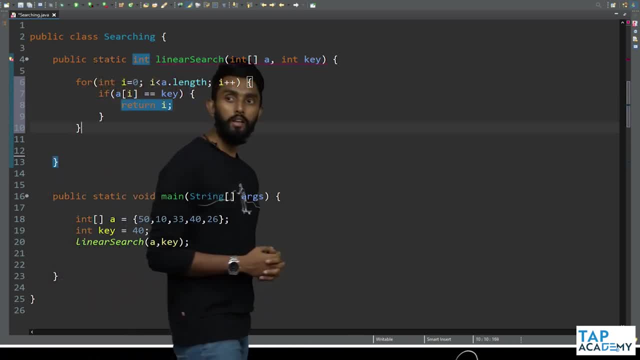 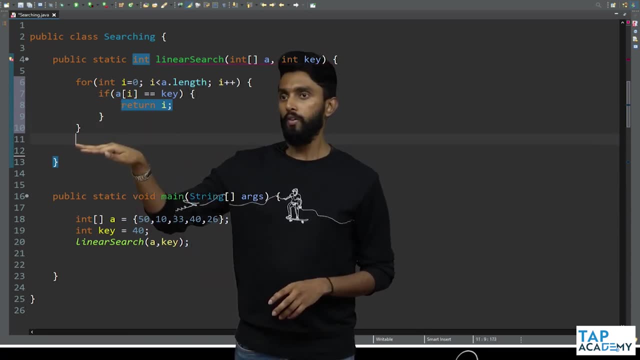 return I And then, if at all, within this during the execution: execution of the loop. this condition never satisfies I will come outside the loop. If I come outside, I know I have not found it, so I will return minus 1, right.